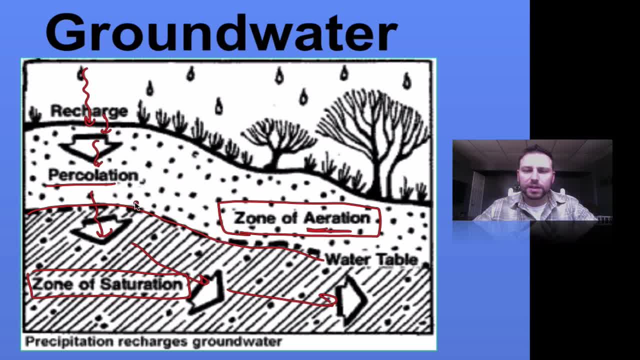 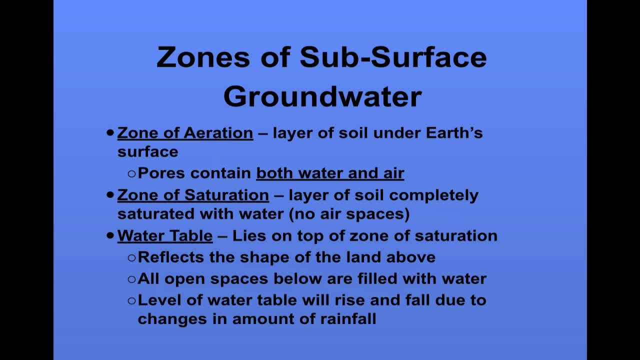 of the land It closely mimics it. I would get this diagram down. it's a nice little diagram to have. So here's a couple of the terms just explained out for you. So we have our zone of aeration. it's just a layer of soil on the earth's surface, but the pores of 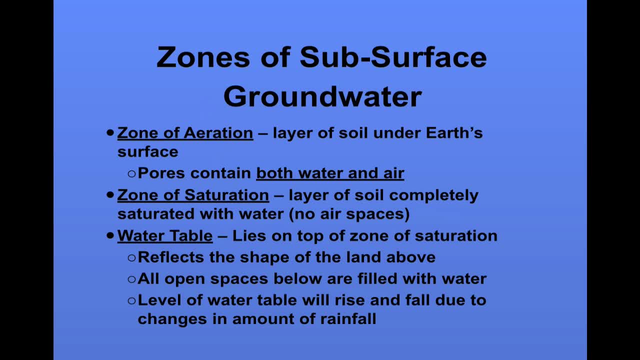 this of the ground contain both water and air. We have our zone of saturation, like I said, that's the soil completely saturated with water and the water table is going to be on top of that zone of saturation and, like I said, it reflects the topography of the land. We could take a look. 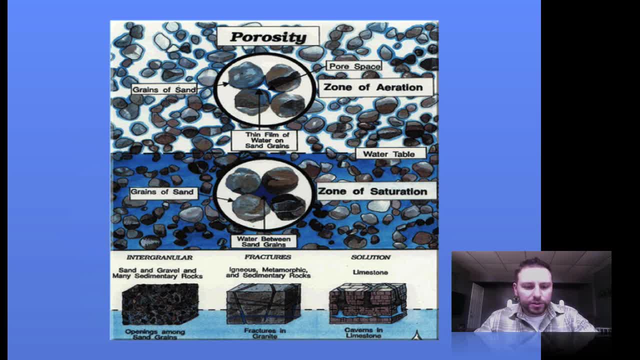 a little bit closely more at the sediments that make up these few different layers So we can see in our zone of aeration we have water that just surrounds those particles and we have open air pockets in them. The pores are mixed air and water. Zone of saturation: no air. 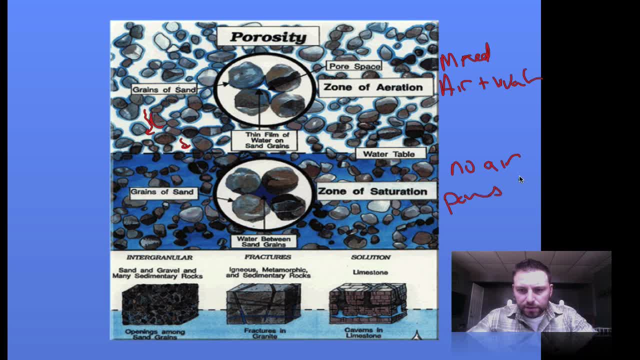 Pores filled with water and our water table lies right on top. So we have a nice little diagram of that zone of saturation. Nice little diagram if you can get it great or make a simplified one like we see with this one and here, that'll be great. if not, it's no big deal. we always have these screencasts here for you to take a look at. 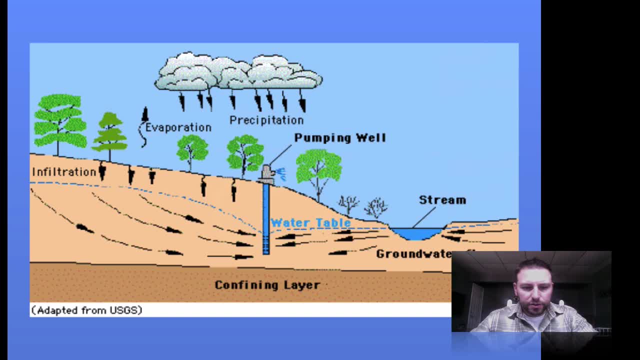 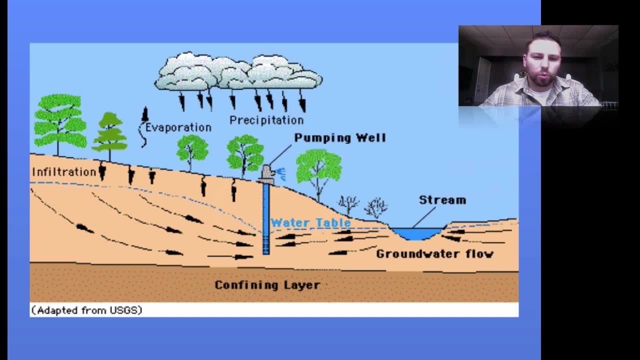 This right here basically is a is a little bit looking outwards a little bit and just how we can have certain features of the land, the water table and groundwater flow. it's a nice little picture of the water cycle also, But we have our water that infiltrates into the ground. 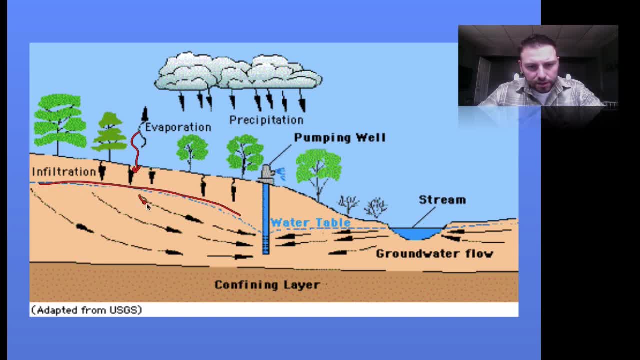 And hits our water table. Notice that the water is following the topography of the land, so goes from high to low, Where it can be intersected by a number of things, for instance a pumping well. you see here, at the pumping well, the water does dip. you'll see in the next diagram that there's a specific name for the dip of water around that well. 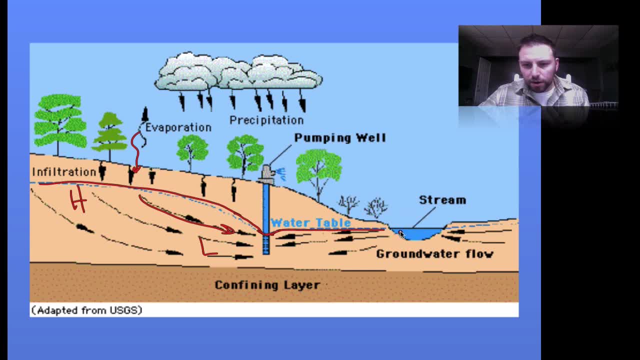 Here's our water table. notice that we have a water table, a stream or surface water that is actually feeding, or that well is actually pulling from that stream. if the well was not there, the groundwater flow would be continuing towards the stream, so we can definitely have a number of different scenarios occurring with our water table.